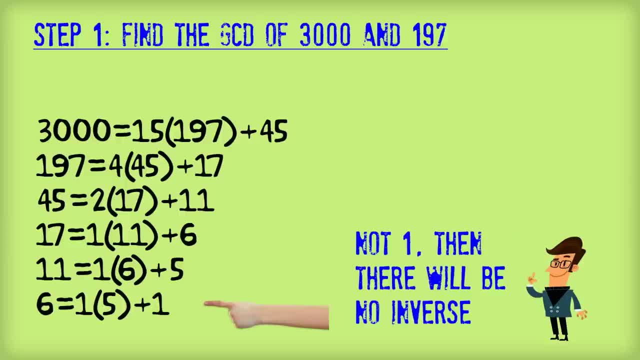 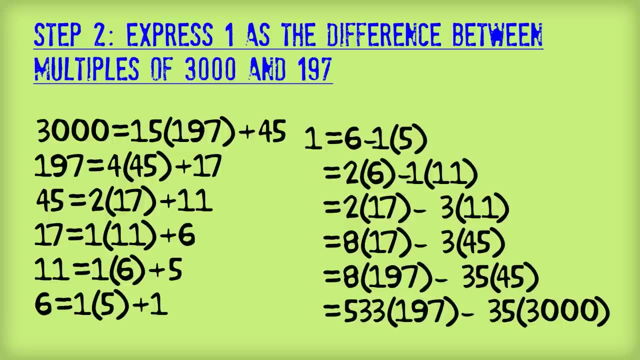 don't get one as the GCD, then there will be no inverse. But in this case we've got one, so we can move over to step two, Which is to express 1 as the difference between multiples of 3000 and of 197.. 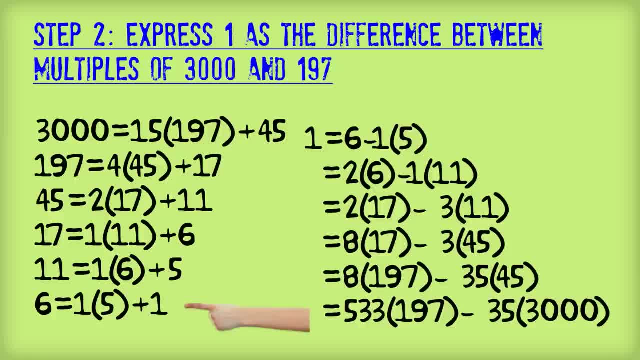 So to do that, we use what we've just done. We start down the bottom here and we can express 1 as the difference between multiples of 6 and 5.. That's just the last line, changed around slightly, And now we want to get rid of the 5, and to do that we look at this line here, which gives us 5 in. 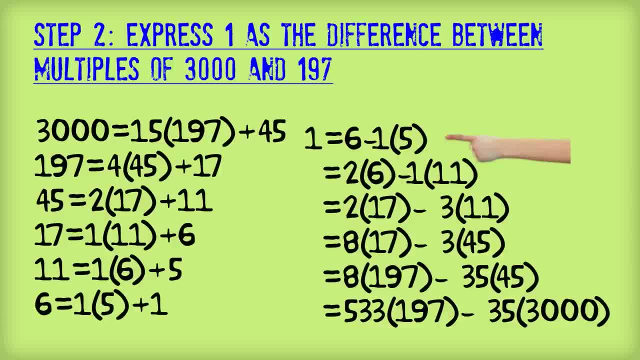 this line here, We substitute that into this, and we get that. Now we want to get rid of the 6. For that we look at this line here, We substitute this line into this line and we get this line. And we just continue this process until we get right down the bottom here, where we have 1 equals. 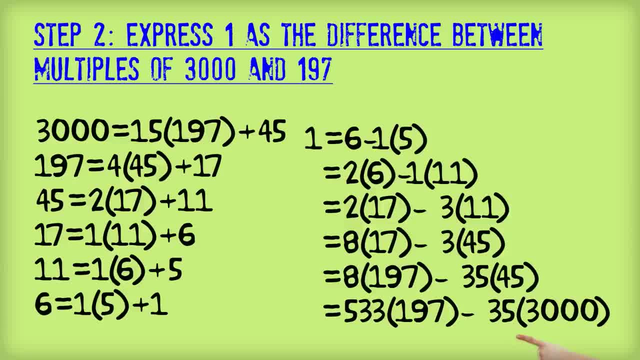 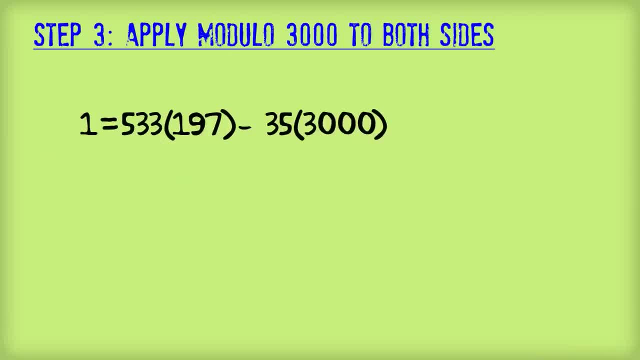 533 times 197, minus 35 times 3000.. Now we're ready for the final step. Step three: Apply 3000 to both sides. So here's our equation. So modulo one on the left hand side is just one. I'm going to leave. 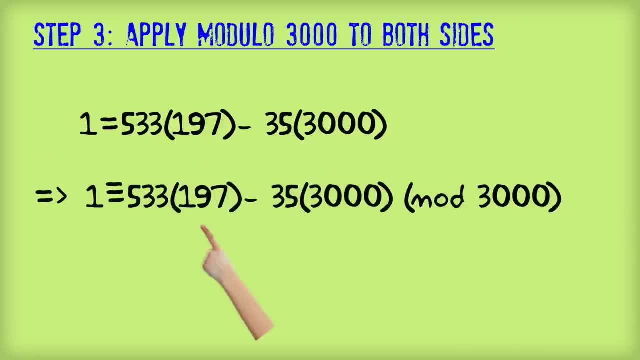 this bit here for a little while, And when we look at this expression here, we see that it's got 3000 in it, and 3,000 mod 3000 is just zero. So this whole expression here is just equal to zero, And we're just left with this. That one is equivalent. 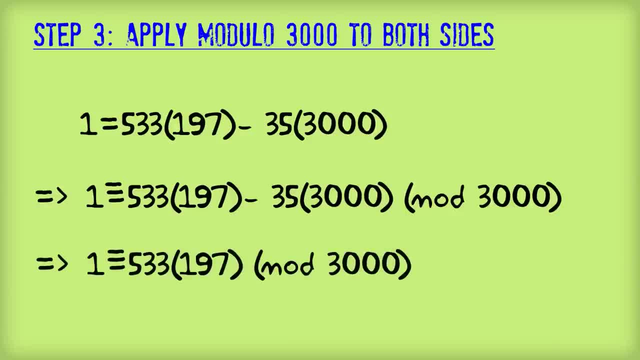 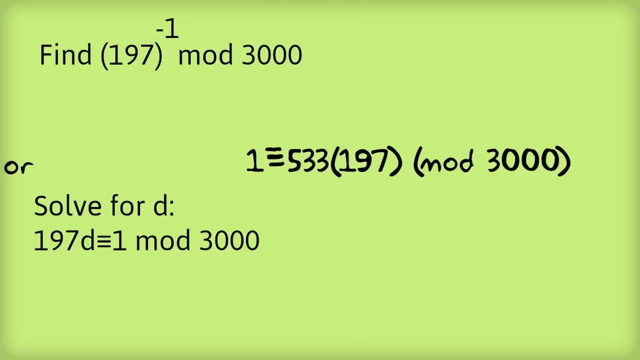 to 533 times 197 mod 3000.. So that means that if we take 197 and we multiply it by 533, we just get 1 in this modulo 3000 world. And that's precisely what we were asked to solve: to work out the inverse of 197.. So here's a way of expressing the answer to the exam. 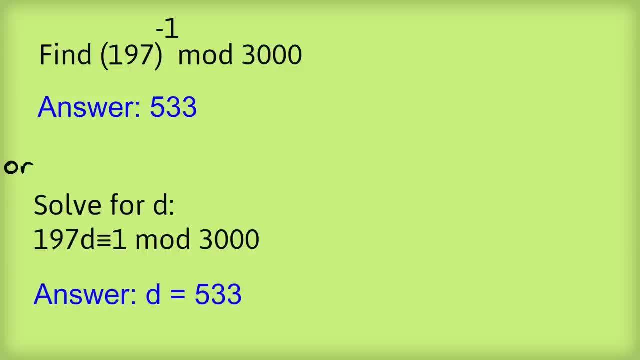 question in this form or in this form, But in either case you should get a green tick because hopefully you'll get full marks. That's it for modular inverse made easy. I hope you found it useful.